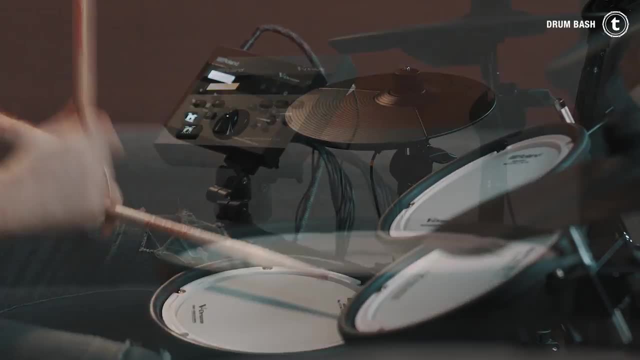 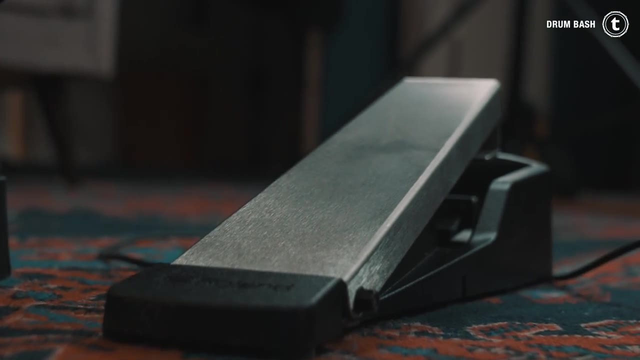 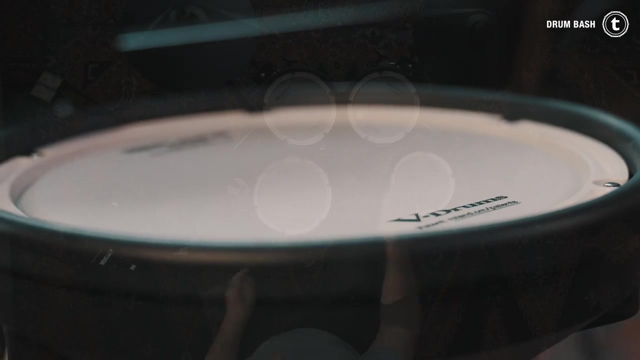 This kit just feels great to play. The translation from the pads to the module is amazing, Especially the hi-hat, which always is the problem when it comes to e-drums. The pads feel a little bit hard though, but the response of the kit while playing faster rolls around. the kit is very good. 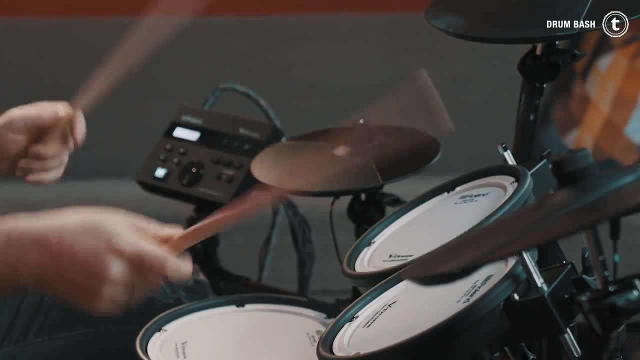 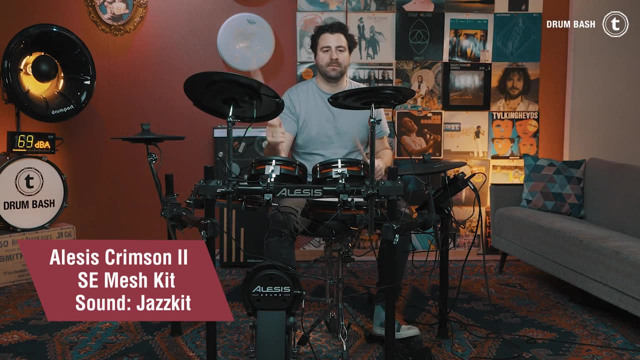 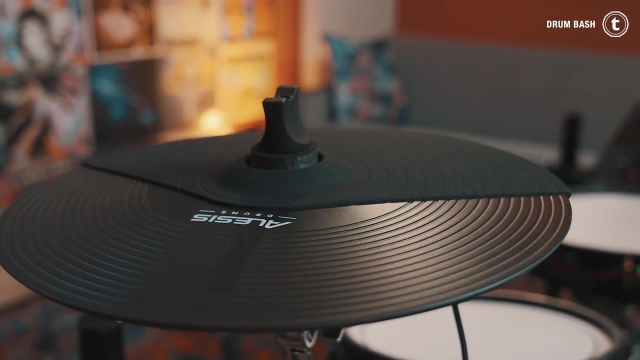 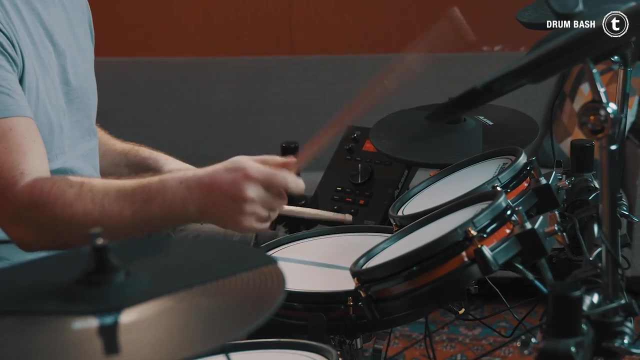 But what about the sound quality? Let's listen to two different sounds per kit: Elise's first. Elise's second. Elise's first. Elise's third. Elise's fourth. Elise's fifth. Elise's fiftth. 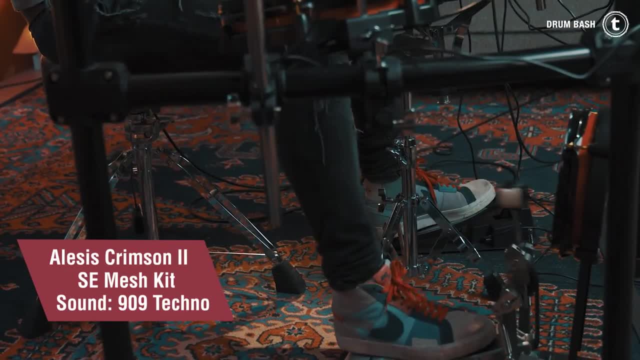 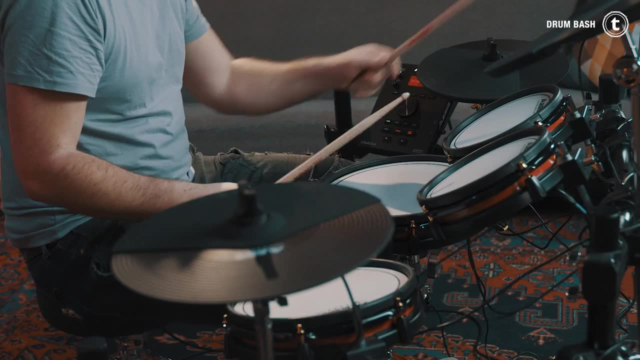 Elise's sixth. Elise's eleventh. Elise's木ed done. Elise's fifth. Elise's sixth. Elise's ninth. Elise's eighth, Elise's twelfth. Elise's chart, Her fiftth. 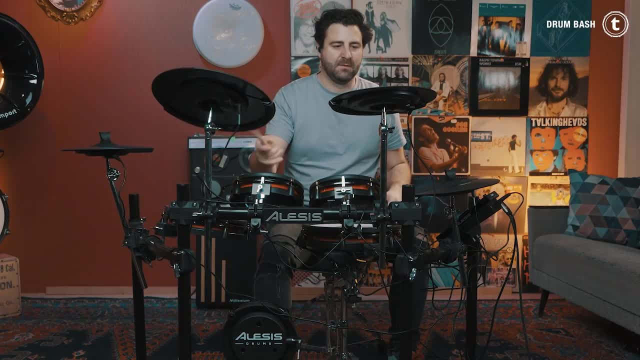 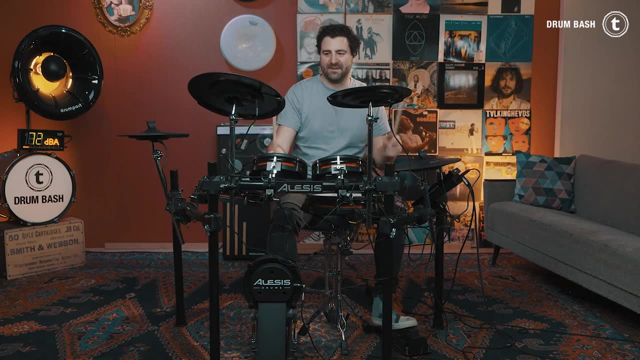 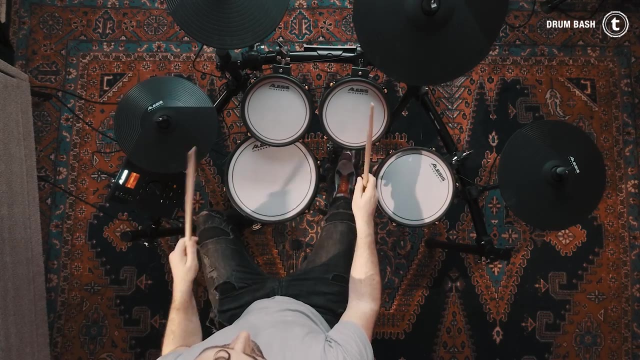 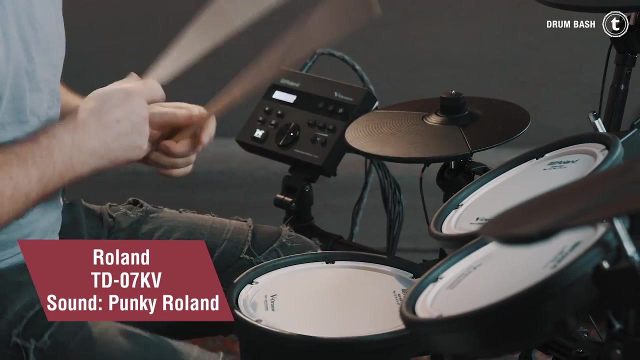 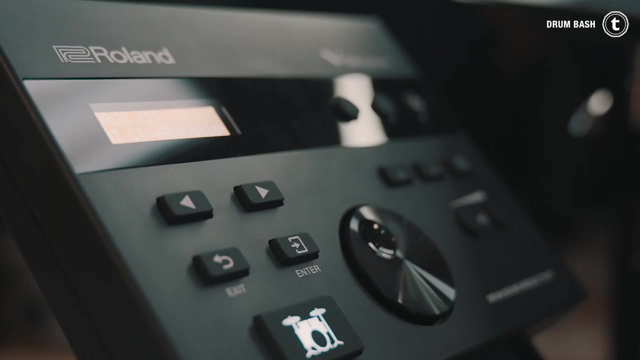 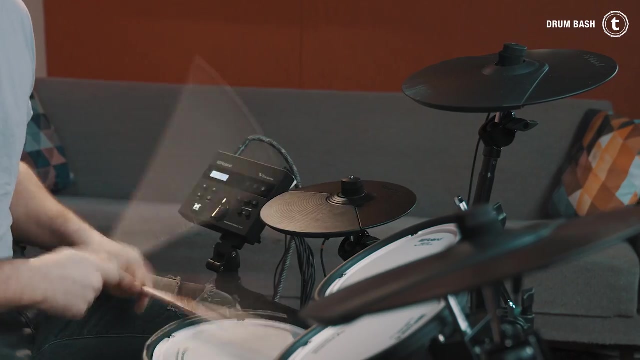 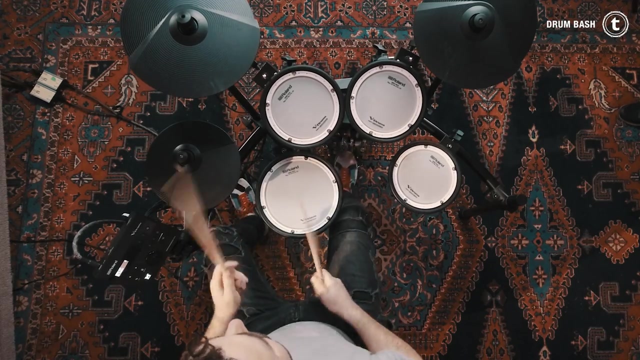 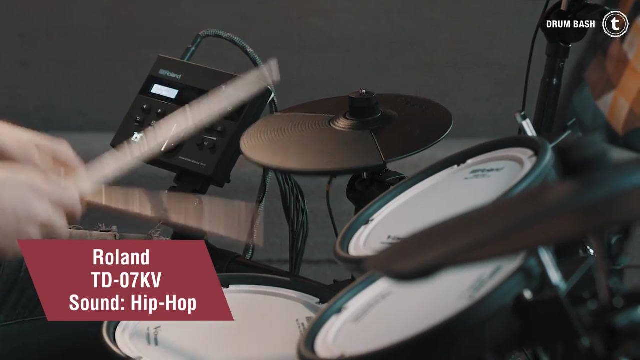 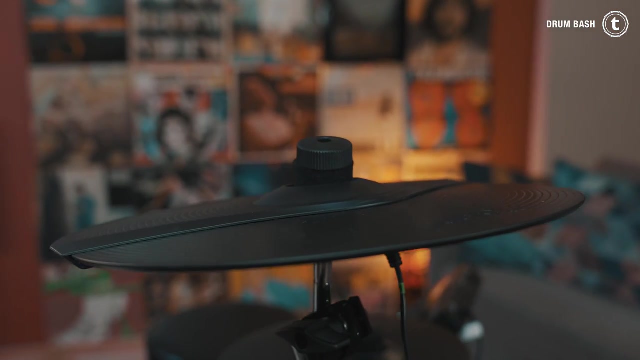 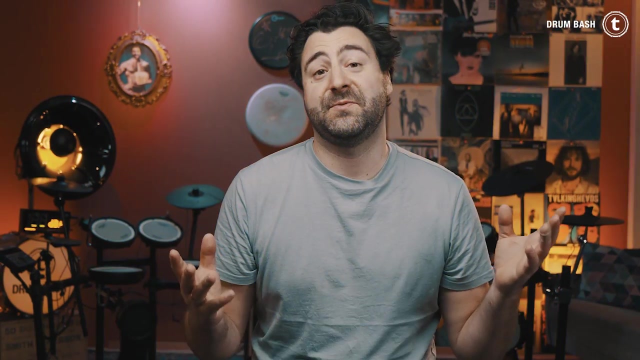 jeunes's sixt, thirtieth, she's twelfth, june e growth high. Thank you, Thank you. Okay, this one's pretty obvious. The sounds of the TD-07 are better than the sounds of the Crimson SE2.. 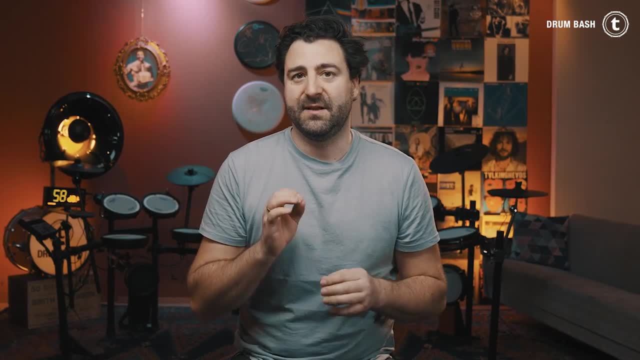 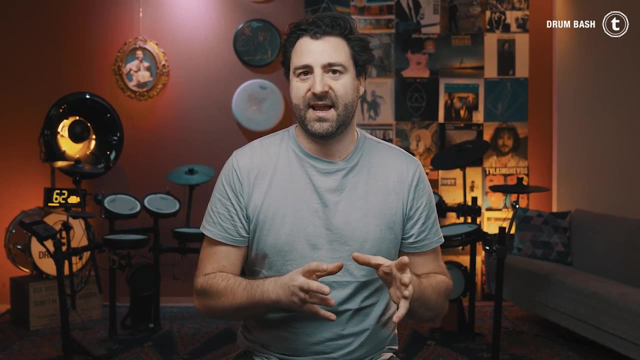 And it's not a big price difference. But with the Alesis you get a 14-inch 3-zone ride cymbal, a 14-inch snare pad on a stand and a 12-inch floor tom pad for less money than the. 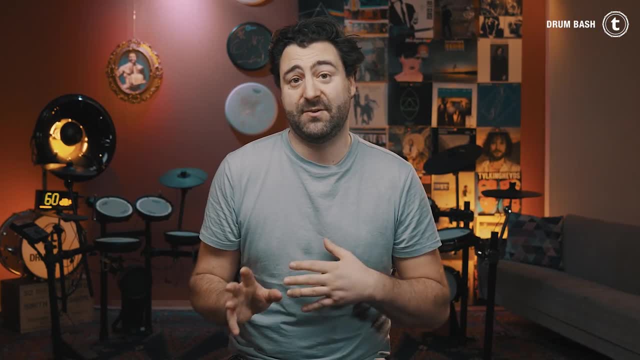 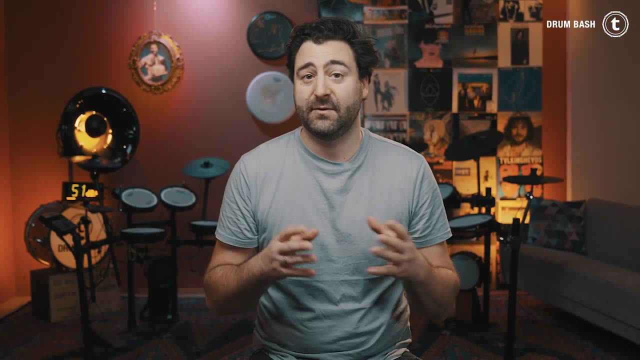 Roland kit. So you have to decide which way you want to go. Either better sounds or bigger kit. The volume within the room is pretty important if you want to play the drums in your flat, So which drums is more likely to annoy your neighbors? 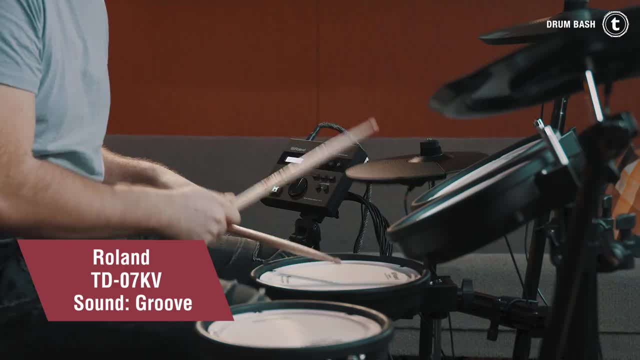 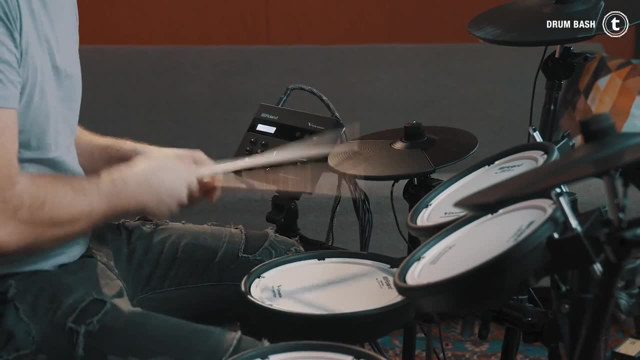 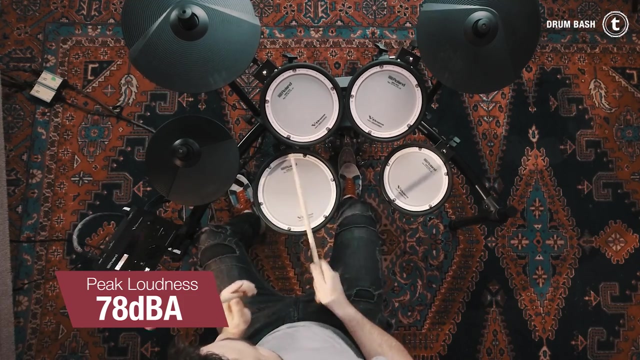 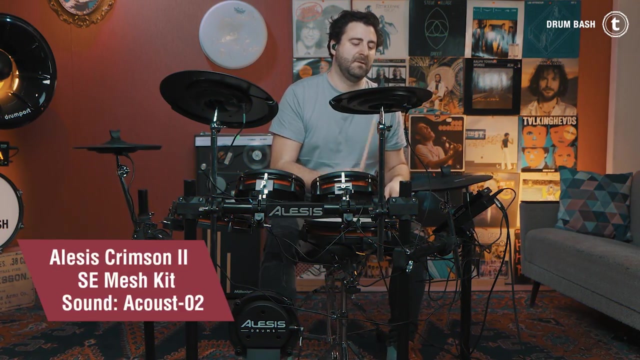 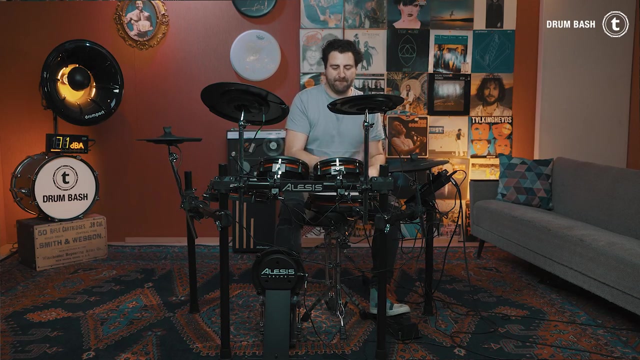 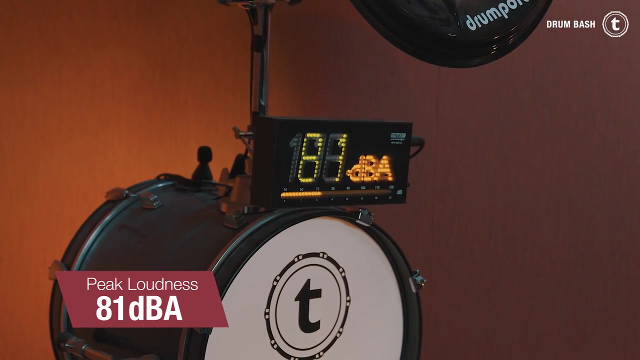 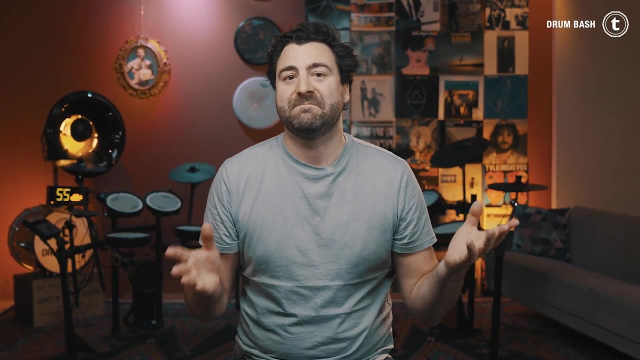 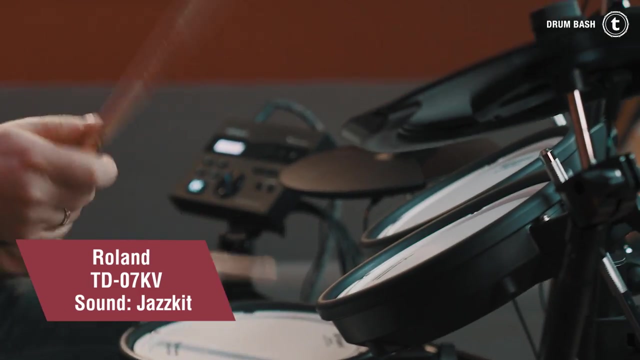 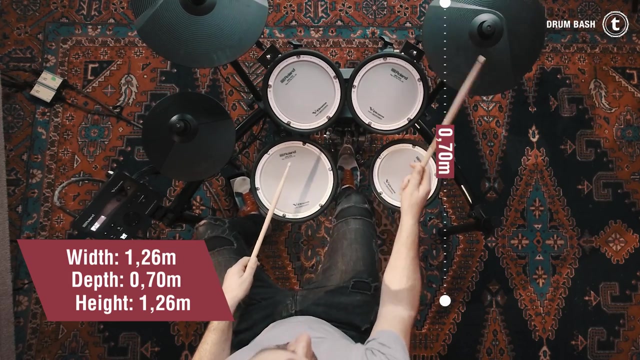 Let's find out, Last but not least, the dimensions of the kit when they are assembled. The Roland TD-07KV measures a width of 126 centimeters, a depth of 70 centimeters and has a maximum height of 126 centimeters. 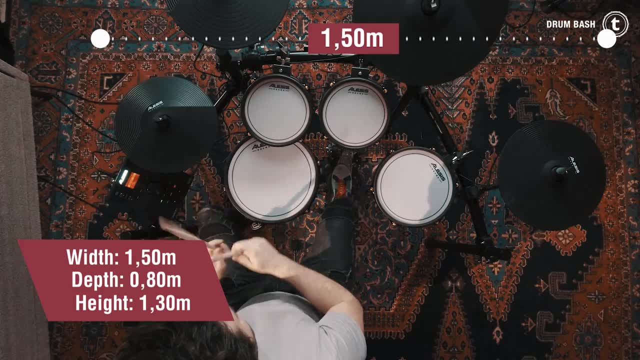 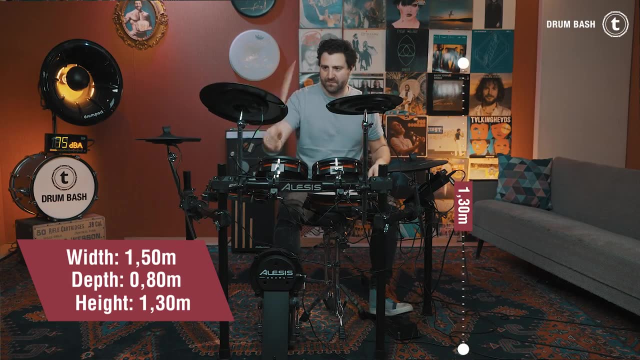 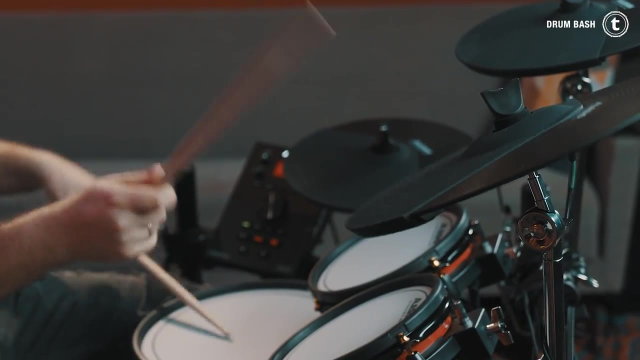 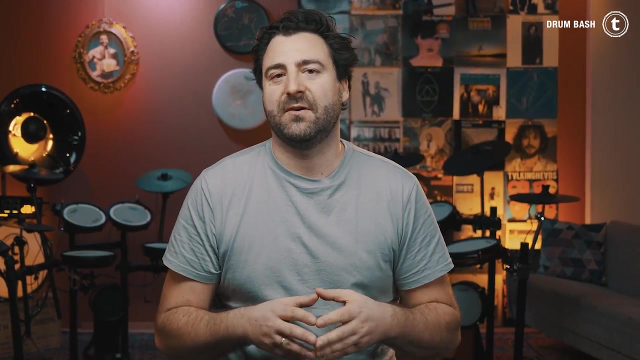 The Alesis, on the other hand, has a width of 150 centimeters, a depth of 80 centimeters and a maximum height of 130 centimeters, So it's quite bigger than the Roland kit. So if you're looking for a more, 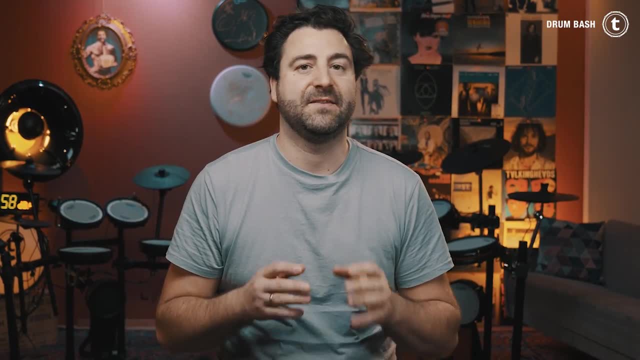 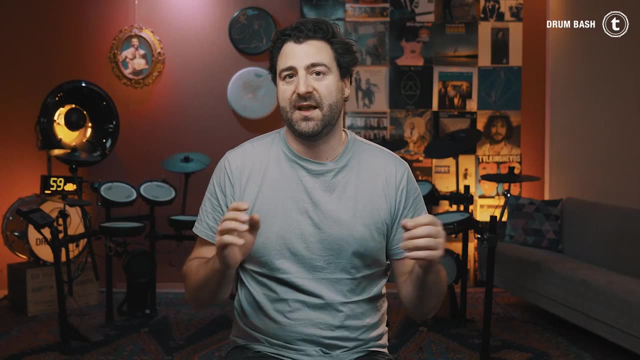 natural-looking drum kit, then the Alesis kit is definitely the right choice. The snare pad on a stand, which is a 14-inch pad, the 12-inch tom pad, the 3-zone ride cymbal and the extra crash goes in the. 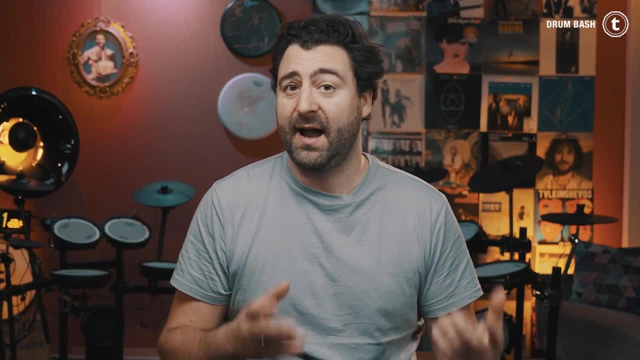 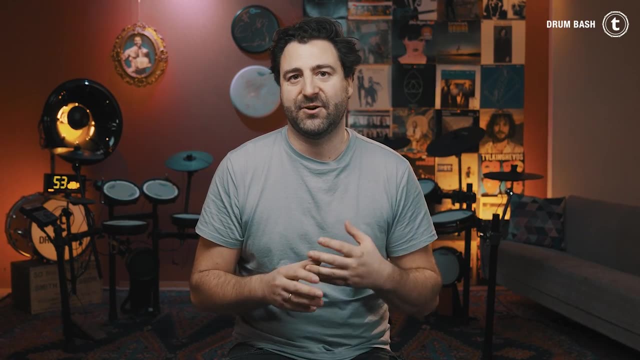 right direction. If you are concerned about the sound quality, then I highly recommend the TD-07.. And the translation from the drum pads onto the module is also better in my opinion, Especially the hi-hat. The hi-hat is actually great, But more importantly, how? 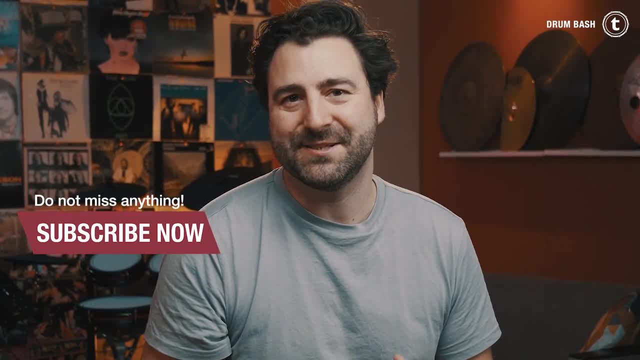 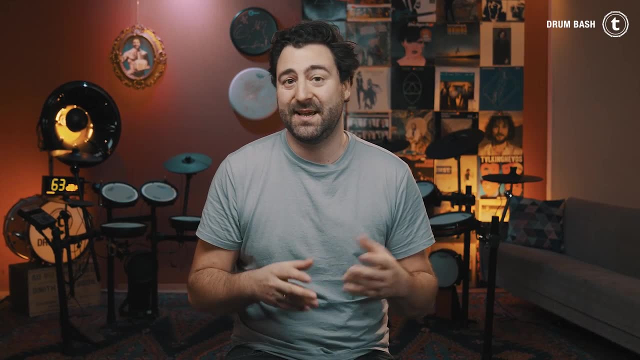 do you like it? I'm looking forward to talking to you in the comment section. That's it for today. I hope you enjoyed this video. If you already subscribed, then I will see you again next week on the Wednesday in a new one. Until then, take. 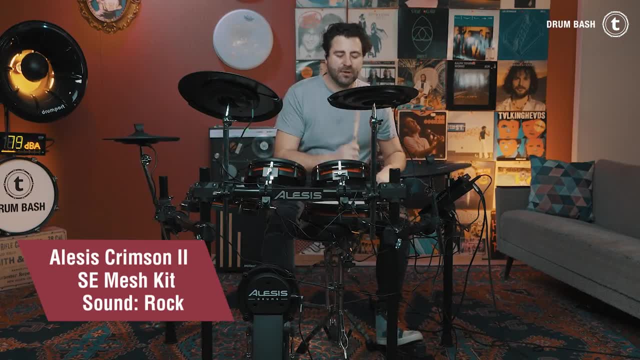 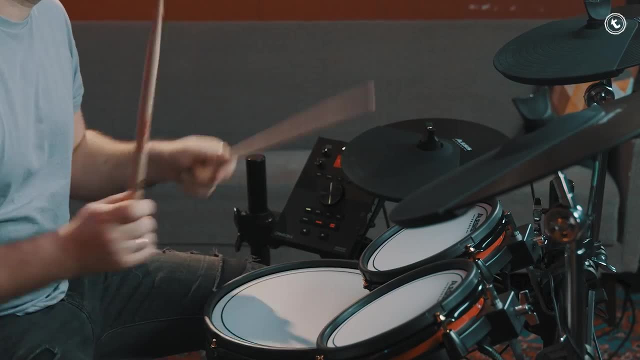 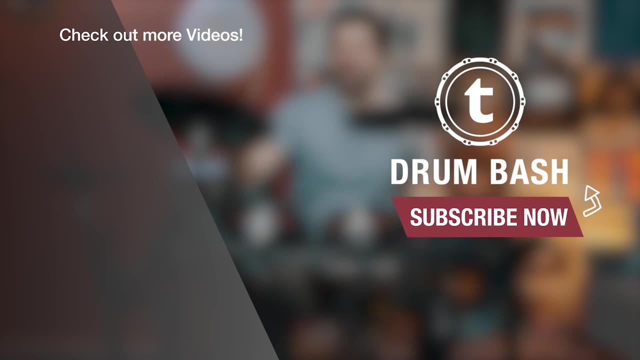 care Simon out, Bye, bye. Captions by GetTranscribedcom.